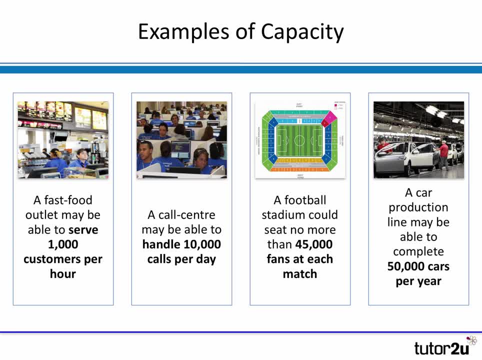 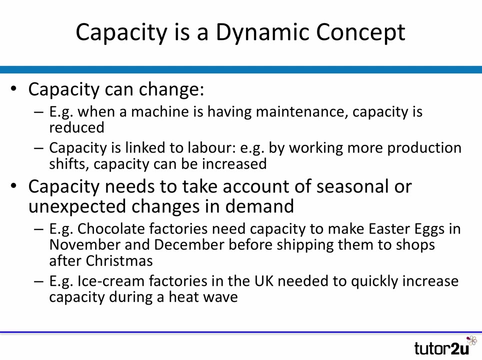 familiar with manufacturing capacity in particular. For example, an example here of the car production line: How many cars could be completed over a certain period? So capacity is a really important measure of operational capabilities. How much can a business produce Over a given period? Capacity is also, importantly, a dynamic concept. Capacity changes, For example, 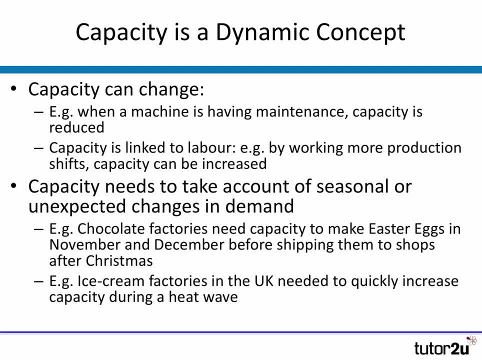 if you've got a production line and you have to repair or maintain or replace a machine, that reduces how much that production line can make whilst that maintenance or repair has been carried out. Similarly, if capacity- how much you can make- is linked to how many people you 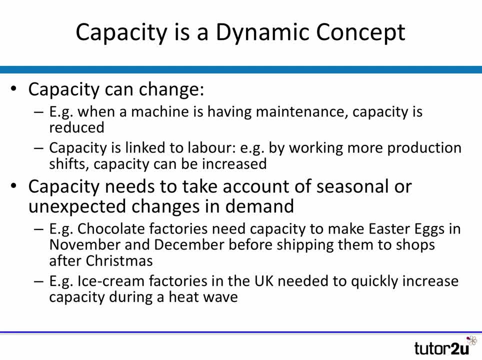 have in the business. your capacity may be affected by how many turn up to work Or how many production shifts that you run each day or each week. Capacity also needs to be dynamic in the sense that it needs to be flexible. Many businesses need to be able to flex or change their capacity to take account of unexpected changes, For example. 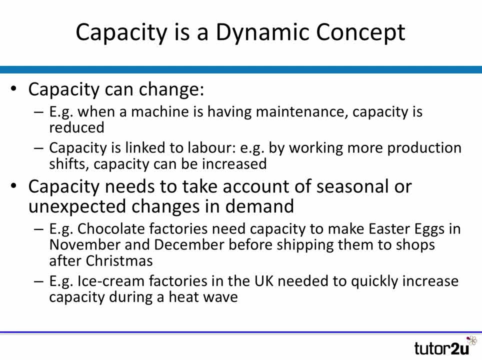 a significantly seasonal demand in a business, You'd want capacity that's flexible, Of course, also picking up on unexpected changes in demand. It's important to be able to add to capacity. So key points so far. Therefore, capacity is a measure of output, It's a measure of capability, But it's also a dynamic 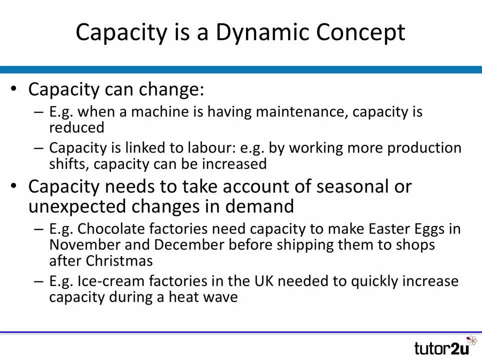 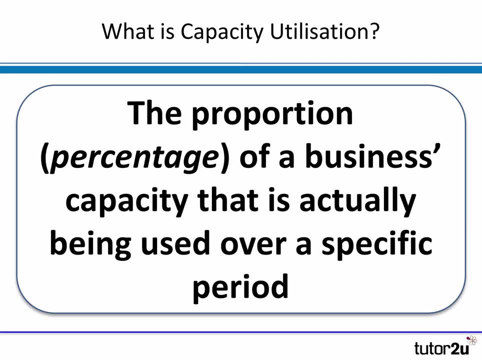 concept, Capacity can be, and sometimes needs to be, changed. Now another important concept of capacity utilization- And there's a clue in the term- The utilization of capacity is how much capacity is used over a particular period, And we calculate this as a percentage. We calculate the percentage. 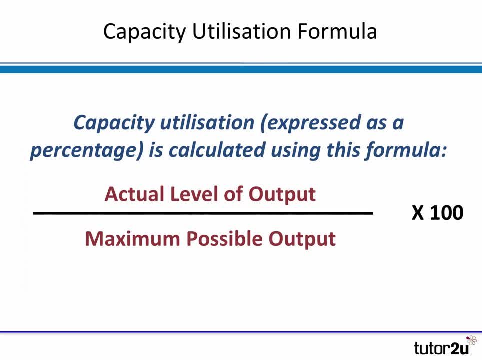 of the actual capacity that's being used. Here's a little example of how we calculate it using this: Capacity is a measure of output. Capacity is a measure of capacity. Capacity is a measure of capacity. So we take this formula. We take the actual level of output, always in units. 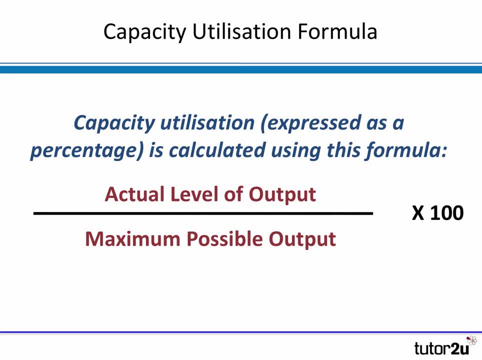 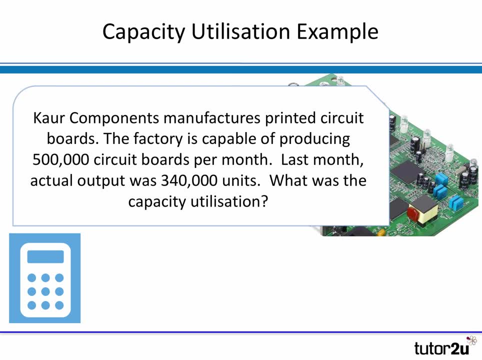 divide it by the capacity, the maximum possible output, also in units, And of course, to get to a percentage, we need to multiply that number by 100.. Let's have a look at an example. In this case we've got a printed circuit board manufacturer, The stuff that goes in so many electronic devices. 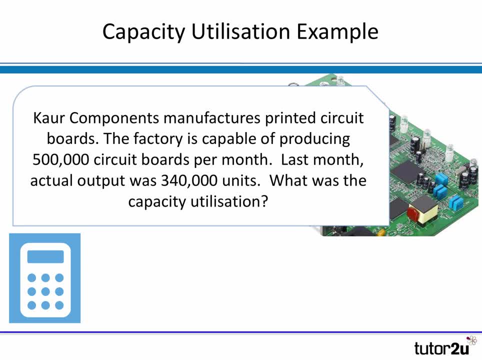 This factory has the capacity is capable of producing half a million circuit boards per month. 500,000 per month, That's our capacity. Last month, we're told, actual output was 340,000 units. What was the capacity utilization? Well, if you want to have a go, pause the video. It's quite a simple calculation Using 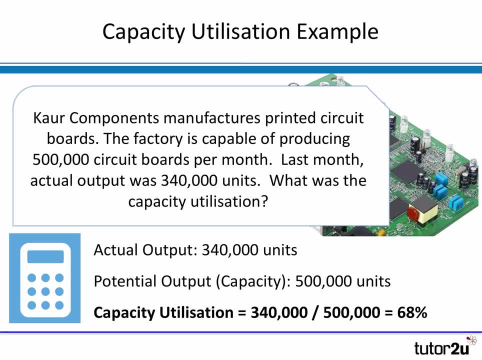 that formula: we take the actual output of 340, divide it by the capacity of 500,000 and multiply by 100.. In this case, that would be 0.68 times 100, or 68%. Now, in a separate revision video, we are: 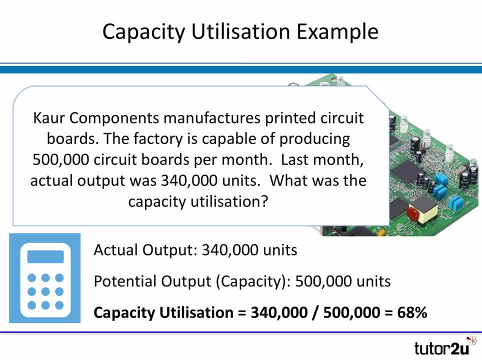 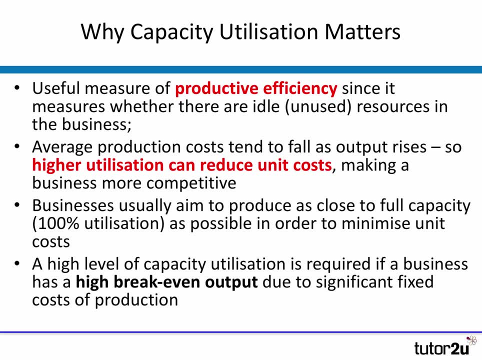 looking at how to calculate the actual output of 340,000 units per month, And we're going to look at how you could calculate capacity utilization in two or three other different ways, But that's the classic way. Now you might be asking why? why are we bothering to look at things like capacity? 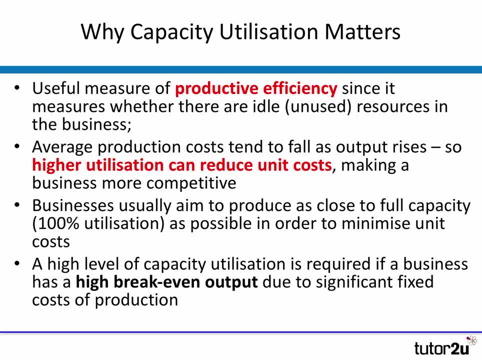 utilization. Well, the key line of analysis here is that capacity utilization is very closely linked to the concept of productive efficiency And therefore it's also very closely linked to the concept of competitiveness. If you imagine capacity is a measure, isn't it? of how much? 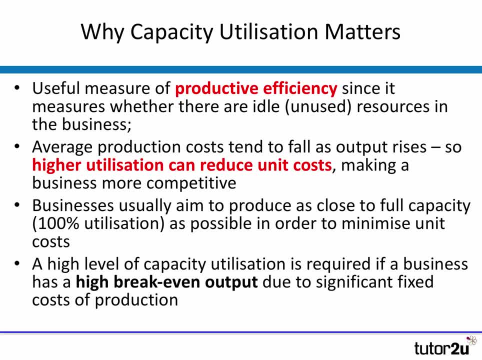 resource we've got to invest in the business, utilization or use of those resources is low. in other words, it has a low percentage utilization. that might be a suggestion that we've either got too much invested in the business or the business is being inefficient. it's got idle, unused resources and, as a general rule, lower. 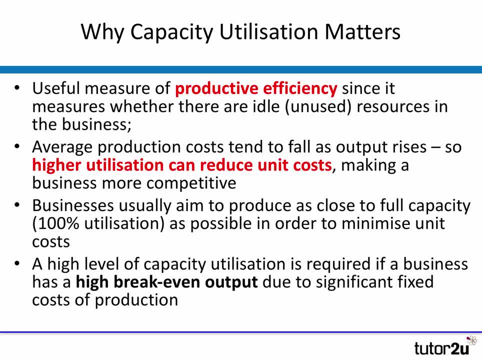 utilization tends to result in higher unit costs because a lot of those resources are fixed costs. so generally businesses try to operate as close as possible to full capacity as a way of minimizing their unit costs, and of course that's particularly important for businesses that have high fixed. 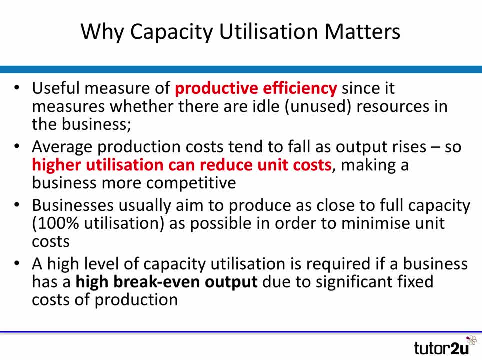 costs because if- if you remember from your breakeven analysis, if a business has high fixed costs, it's important to try to achieve the high breakeven. output and capacity utilization, of course, is a very important part of the business, so that's why we've got a lot of business that. 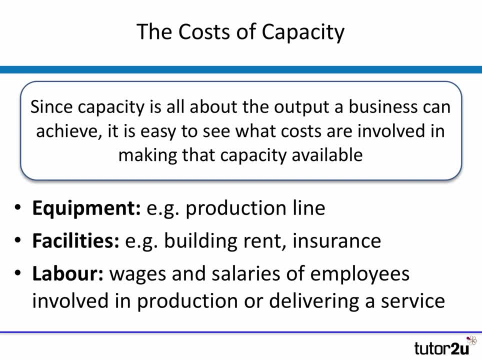 have high fixed costs, and capacity utilization, of course, is a very important part of the business- is going to be fundamental to achieving that. now, capacity has cost. we've talked about fixed costs here. if you think about capacity, it's the way the business enables itself to produce units. 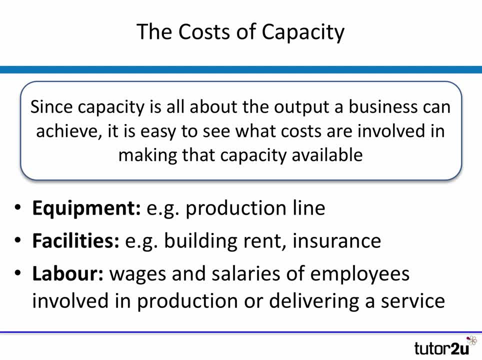 so it's the costs that are involved in making capacity possible. so it's definitely things like production line equipment or facilities, isn't it equipment, facilities, machines and the buildings in which those machines and facilities and services are housed. but of course also that significant cost of capacity is labor, particularly for labor intensive businesses where output 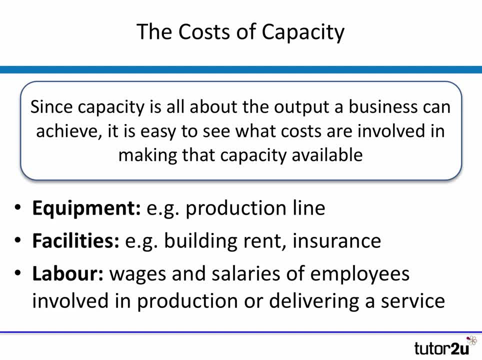 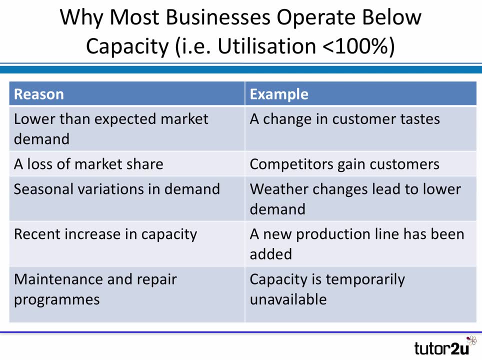 is largely determined by how many people you've got in the business and by how skilled and productive they are. so capacity is very closely linked to the costs of a business. so why, you might ask, would not? would a business not operate at full capacity for as long as it can? 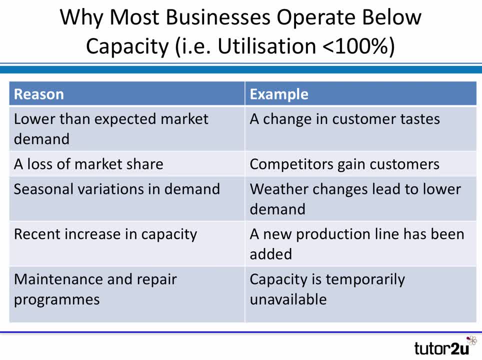 well, the answer is: there are lots of different reasons why it's not possible to operate at full or 100 percent capacity. so the answer is: there are lots of different reasons why it's not possible to operate at full capacity for as long as it can. well, the answer is: there are lots of different reasons. 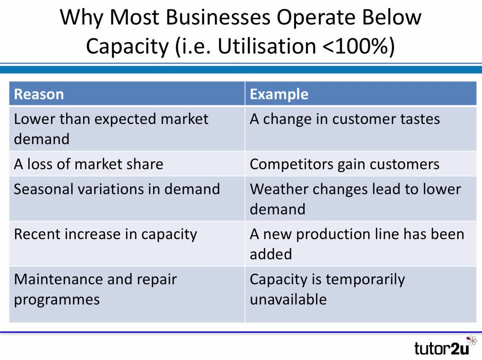 utilization. firstly, of course it might just be that demand is lower than you expect. so you've got a factory that can sell a hundred thousand units, but demand is only fifty thousand units. well, there's no point running the factory producing a hundred thousand if the demand isn't. 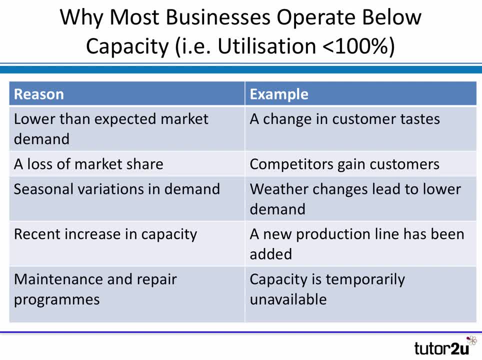 there. so lower than expected market demand can reduce capacity utilization and of course, that might also be a symptom of a loss of market share. maybe you used to be the market leader with a large factory that was very busy. you lose market share. all of a sudden, the large factory is still there. 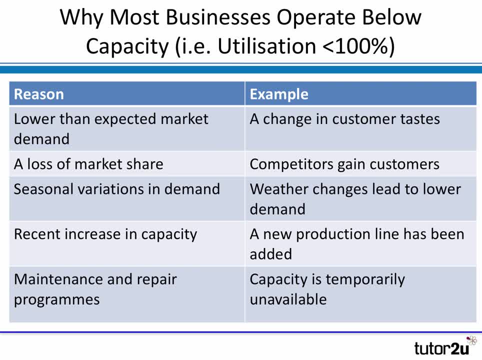 but you're not so busy. we've also mentioned, of course, these. there can be these seasonal variations in demand that can affect utilization from from month to month or week to week, and of course, it could be that actually there's been a recent increase in capacity but not yet an increase. 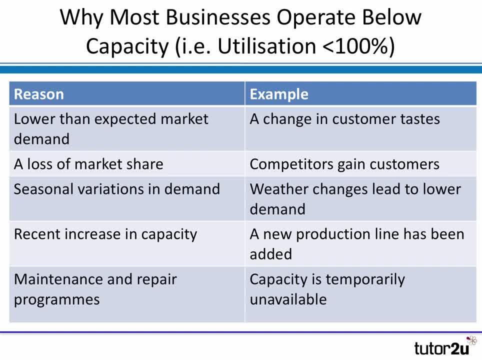 in demand, and that would be a reason why utilization is less than 100%. but of course, generally you can't really achieve 100% because of the need to maintain and repair your capacity. there's always going to be some parts of it that just needs fixing or repairing or maintaining, and 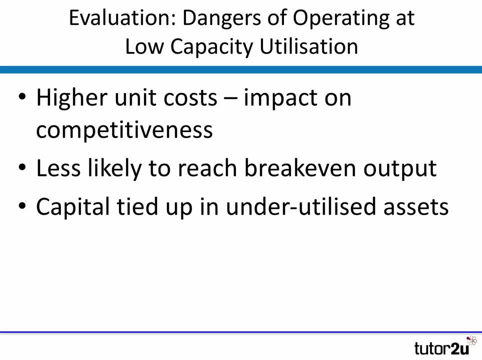 a quick bit of evaluation to finish off. a classic question might ask you to consider the the risks or dangers of operating at low capacity utilization. what might the implications of that be? well, I think we've already hinted at this, haven't we? which is that low capacity utilization, particularly for a